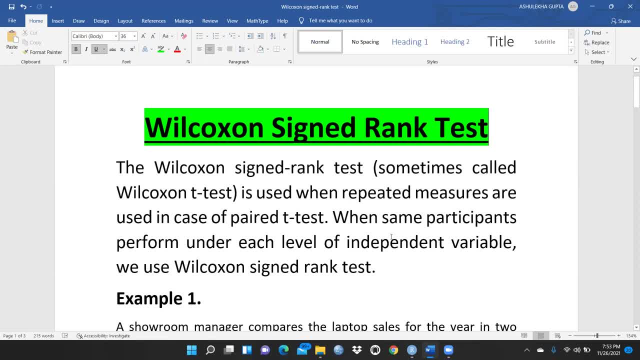 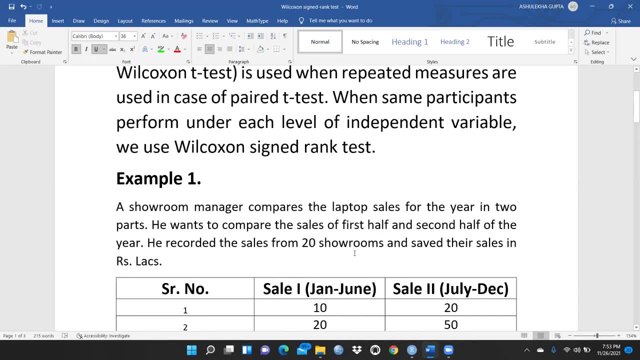 independent variable. we use Wilcoxon signed rank test. So here is, I have got the data. a showroom manager compares the laptop sales for the year in two parts. He wants to compare the sales of first half and second half of the year. Here is the sales of first half and second half of the year. 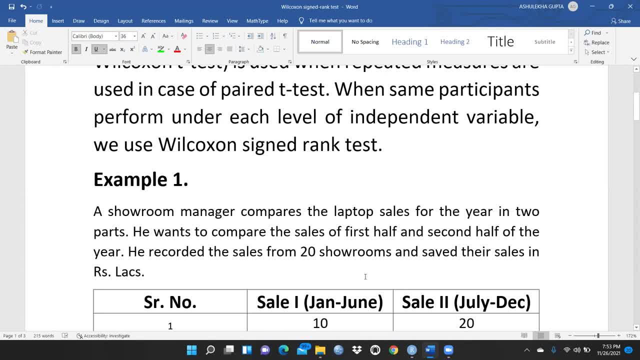 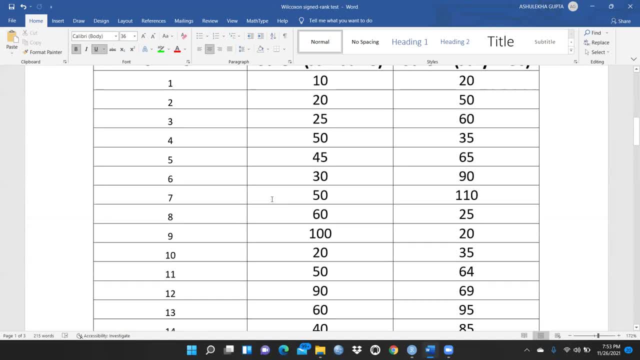 Here is the sales of first half and second half of the year. He recorded the sales from 20 showrooms and saved their sales in rupees legs. So here is you can see serial number I had mentioned total 20, sample size and sale one means that is the first half. 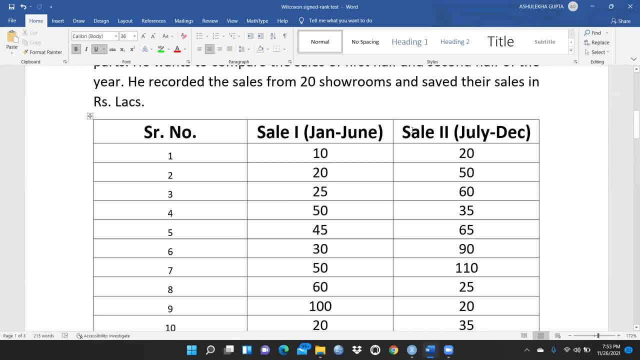 year sales then to June and sale two July to December sale. So here is we want to just check, we want to compare whether there is any significant difference between these two. the. this is the biannual data, So there is any significant difference. So let me I had created 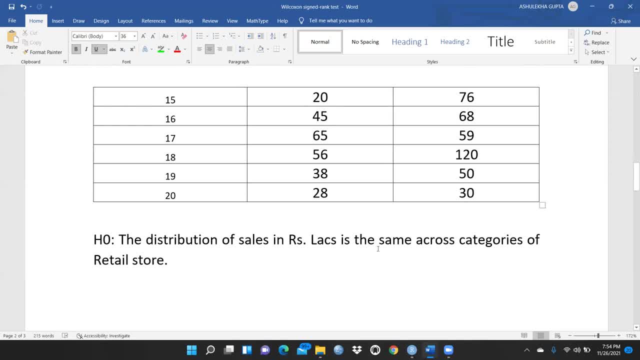 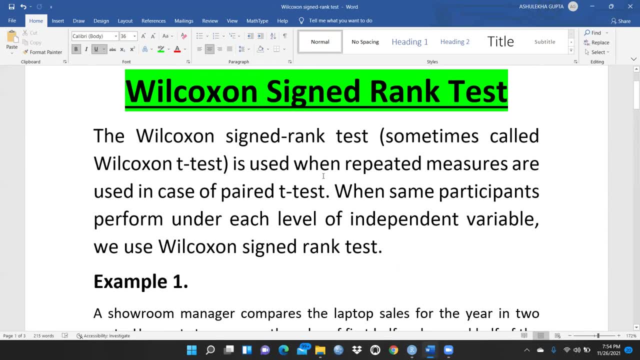 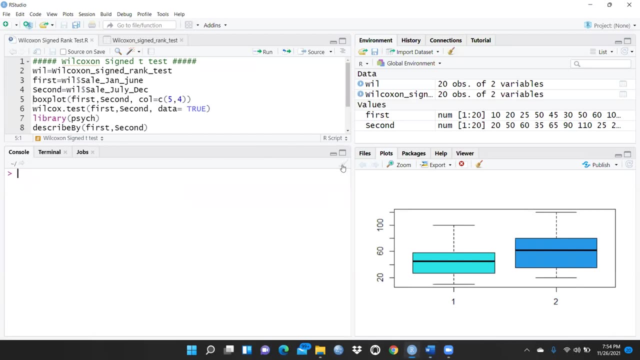 this hypothesis, the distribution of sales in rupees legs is the same across categories of the retail stores. So we have to check this data through our studio, through our. so let me clear all these things. I would start at fresh. I am clearing all my windows. 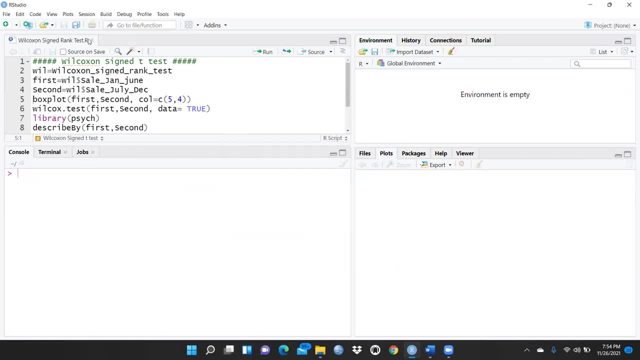 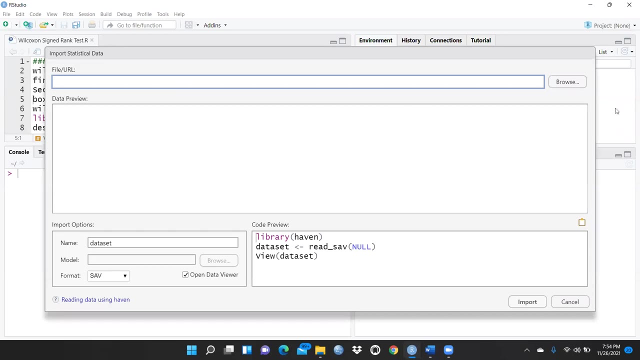 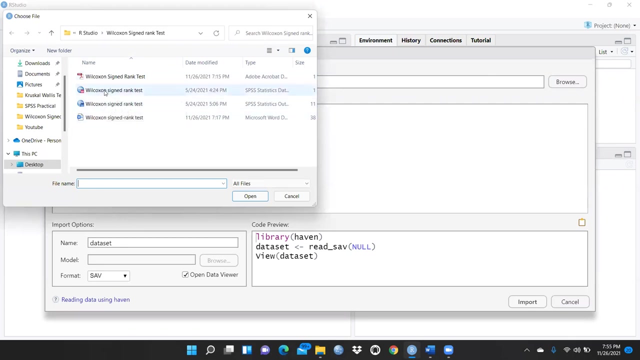 Yes, and I am closing this file also. and now you can see this is the R script. and now what we have to do: let me open, let me import my file. My file is. I am going to. I want to import my SPSS file. Let me browse it and this is my SPSS file. and let me open this file and I am going to open. 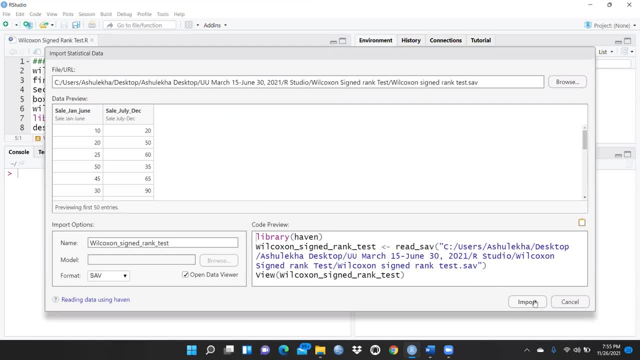 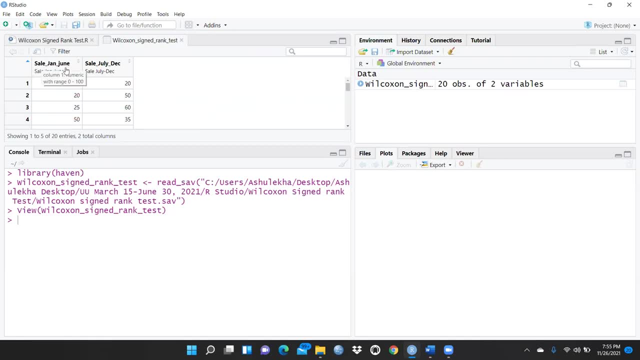 this file and i'm i want to import this file. let me press import. and now you can see here: here there is two columns: sales gen to june and sales july to december. so now you can see how many entries are here. total number of entries are 20 and that is reflecting also here wilcoxon sign test and 20. 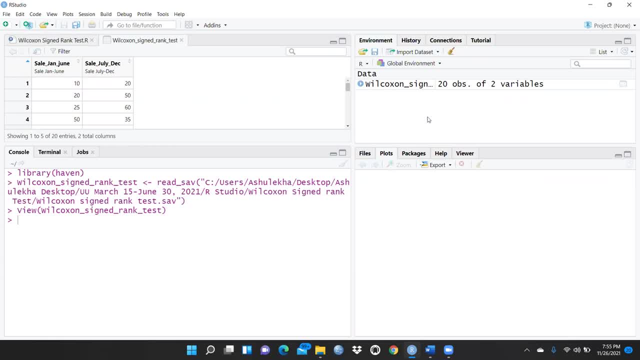 observations of two variables. so i am carrying only two variables, but there is 20 observations are here. so let me start first of all, what what i have to do. first of all, i would like to put this file in our variable. let me create, because again and again, i'm not going to use this is the very 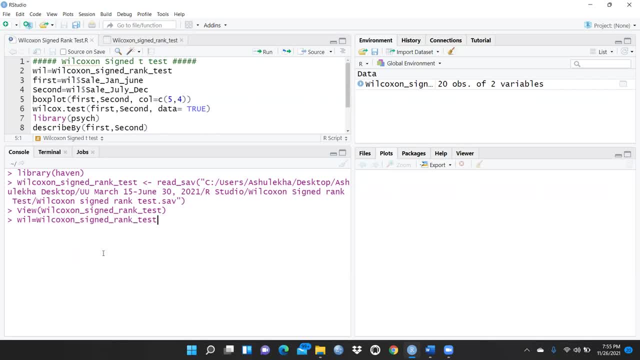 lengthy name, so i'm just wilcoxon sign rank test. this is my file name, so i'm i am putting this file in this variable, so let me enter. and now you can see: this variable is created here: wil and 20 observations of two variables. so what we have to do again and again. i'm not going to use dollar sign, so what i am. 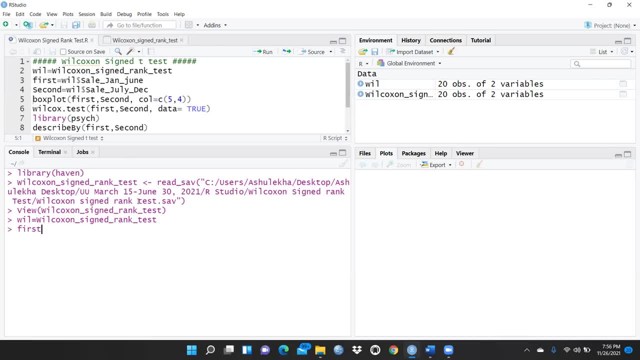 doing? i'm simply writing, i'm i'm just, i'm just putting up because i am carrying. i'm having these two variables. this one is the sales gen to june. so i'm creating this, the one variable, first, where i will put this data, and second, i have to put this data. so what i have to do first, let me 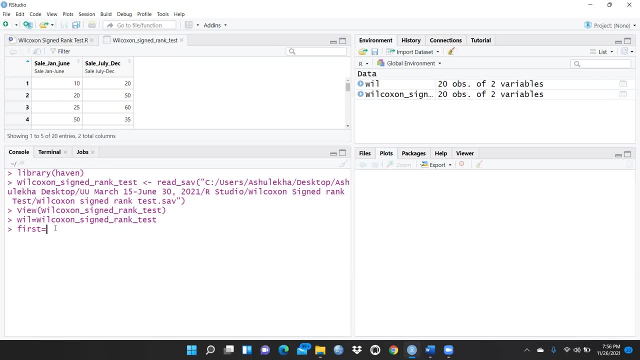 and where this file, the this, this, these variables are putting. i'm writing just w, i l will. this is my file name. then i have to press dollar sign and sales gen to june, because this is my first year, first half sale, so i will press enter. so now this variable is created here and now again i would like to create variable. 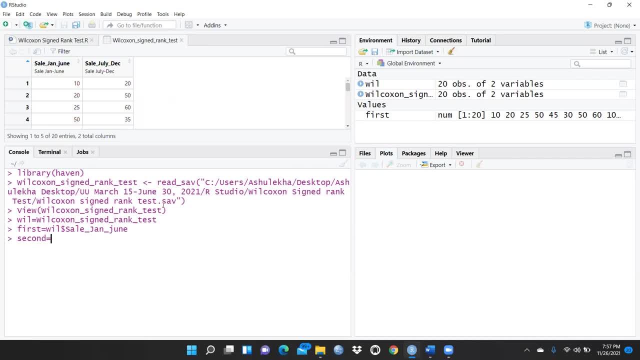 second and when i'm writing second, and now you can see simply this variable is put in here and i'm putting where here is will, right, this is the file name, and simply i will put dollar sign and the next half we have to put there. so now you can see both these variables are. put it here, right? so what? 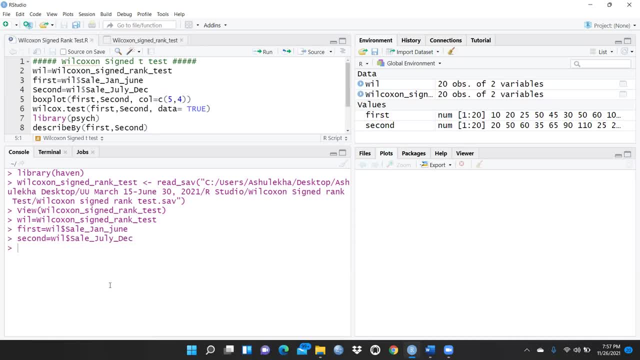 we have to do. you can see now. uh, simply, we want to check whether our data is sorry, data is normally distributed or not. so, simply, i would like to just check through box plot and, uh, what i have to do. i had already put it first, because this is my data, that is. 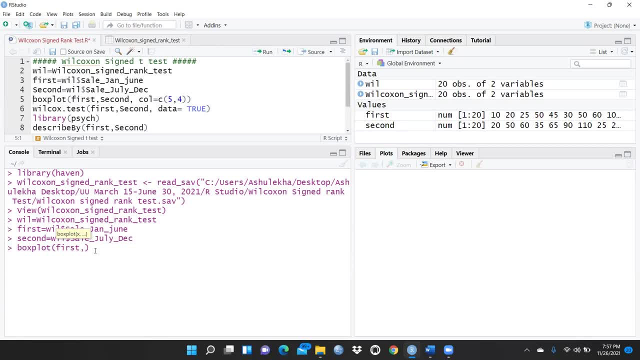 january to june and then july to december is my second. i had already created these variables, so i have to put this data and i would like to give them some color schemes also. so here is colour scheme. i just want to give, let's say, three and four, so i have. 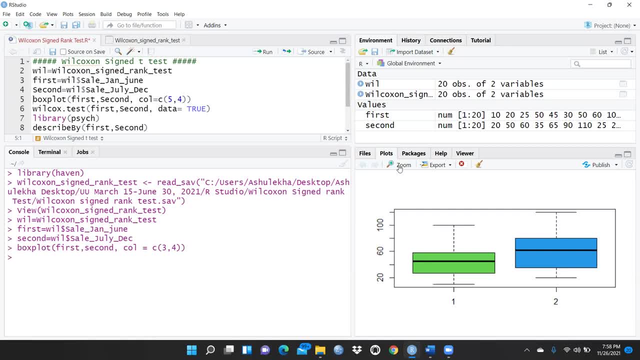 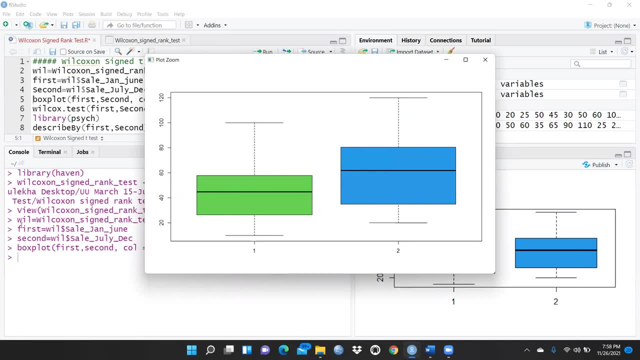 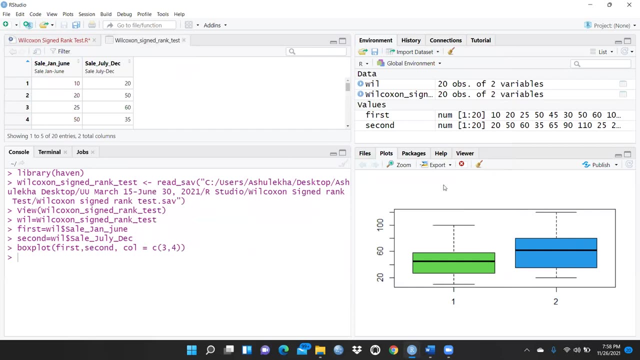 just press enter. so now you can see. these are my two box plots are available here. that is for one, that is for two. one means that is the first, right when we are comparing this data- sales june to june- and second is sales july to december. so what we have to do here is you can see this is the i mean. 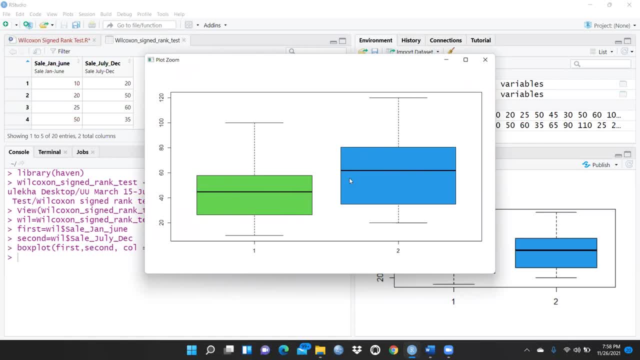 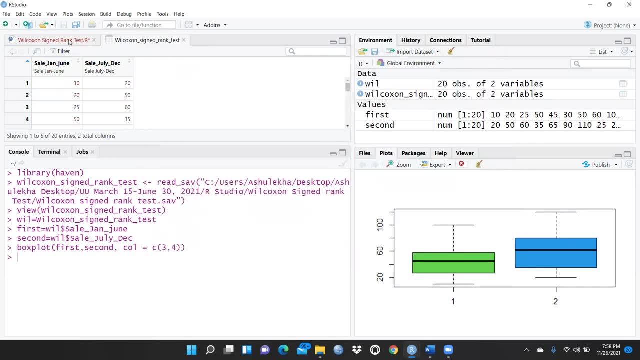 this is the mean value and this shows what is the difference between both sort of this data. so what we have to do now: we want to check this data, right, we would like to apply wilcox, and sorry, here is i just want to apply this data. on this data we want to check, i would like to apply. 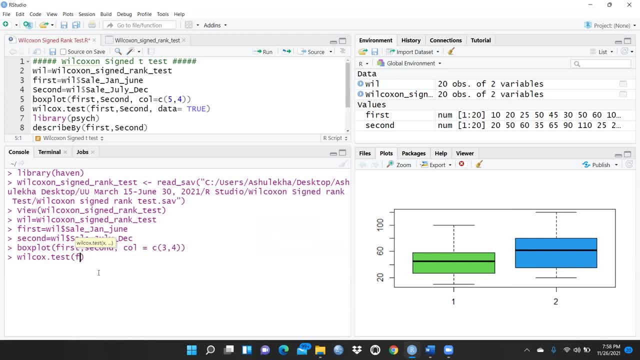 wilcox test and what we have to do. simply i have to write first and i have to write second, because both these data and what i have to do- let's say i I'm writing when data equal to, I'm just writing data, or simply we have to use paired right. 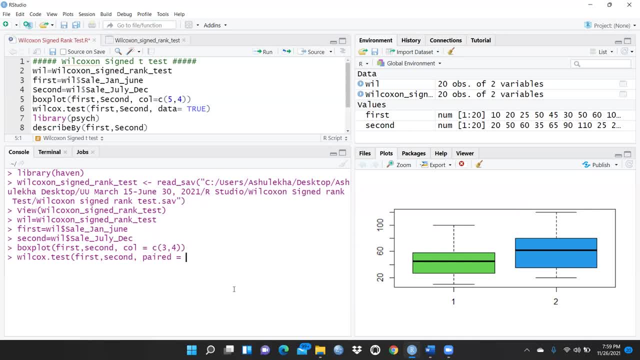 paired. When paired is equal to true, True means true means yes. this is the same sample and that is some kind of pre or post kind of test. If you would like to write otherwise, automatically what it would by default: that would be false. If you are writing false, I will show you how you. 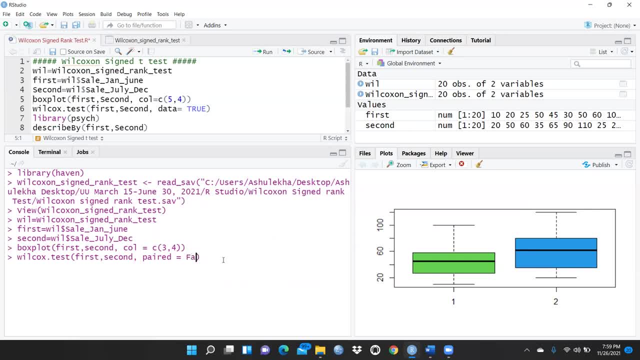 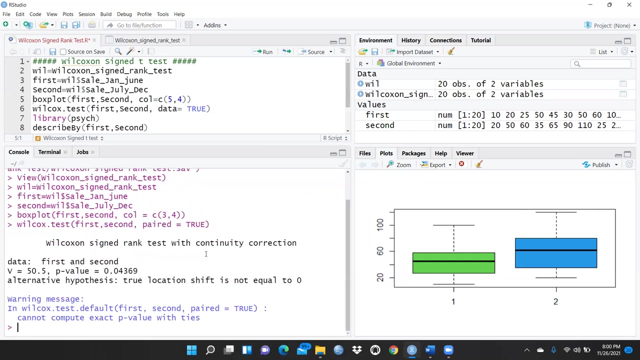 have to write If you would write false here. so that means there is no pairing. That means both these datas are two independent data, first and second. There is no pairing, But when we are writing, that is paired, sorry, Paired is true, So that means my data. that is same data where we want to check their difference. 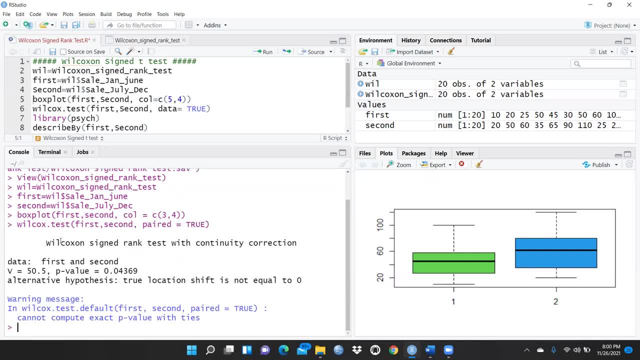 significant. whether they are, there's a significant difference or not. So Wilcoxon sign track test with continuity corrections Here is: you can see V is 50.5, P value is 0.04369.. So that means it shows. In my case my null hypothesis is rejected because my P value is. 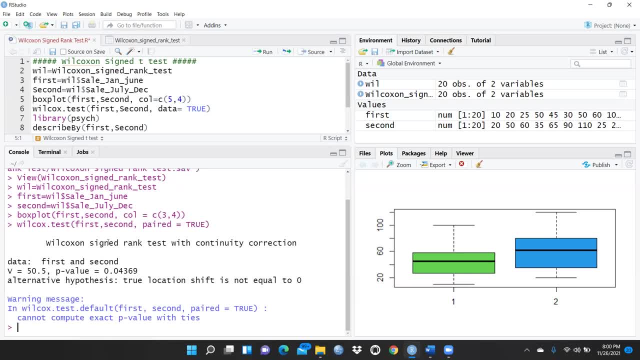 less than 0.04369.. So that means it shows. So that means it shows. So that means it shows And alternate hypothesis is accepted. That means we can say: in my data here is, in the first half and the second half these values are significantly different. That means there is difference in the 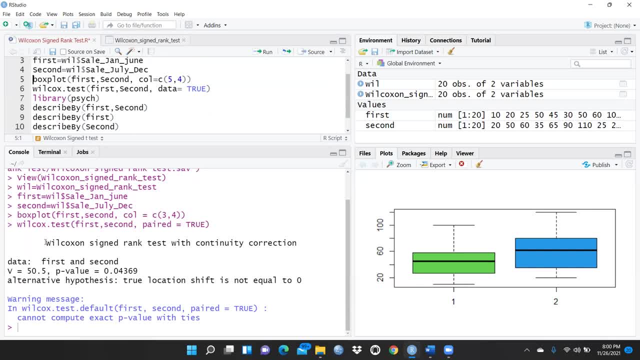 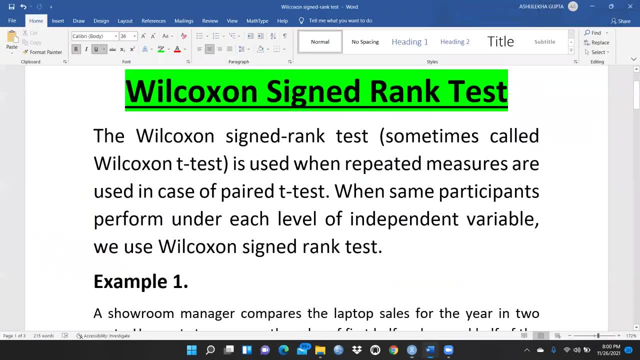 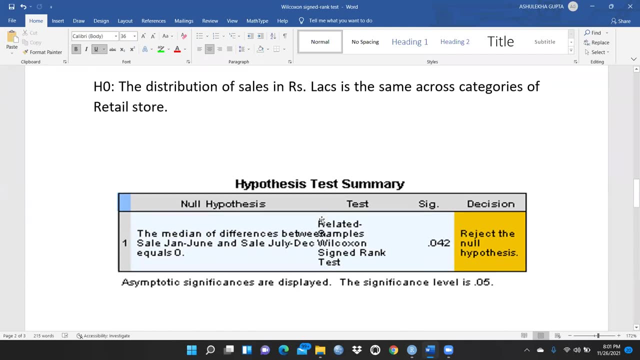 sale across the year. So now what we have to do, we want to check through median also because there is the. I had written one statement That was my through SPSS. I had already shown and you can see here this is my through SPSS. 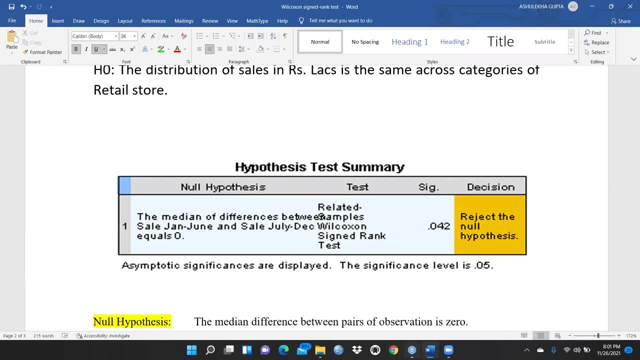 and the same results we have got through R also. So here is you can see 0.043.. And when I had applied this, the same data through SPSS that was 0.042.. And we had rejected the null hypothesis. 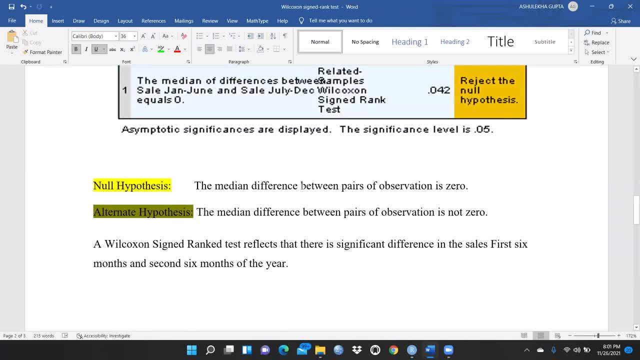 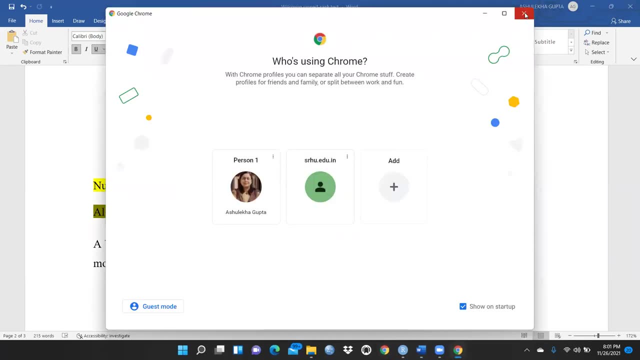 but through median. null hypothesis, say, is the median difference between pairs of the observation is zero, But alternate hypothesis said the median difference between the peers of the observation is not zero. So what we have to do simply, I would like to apply this median test also. 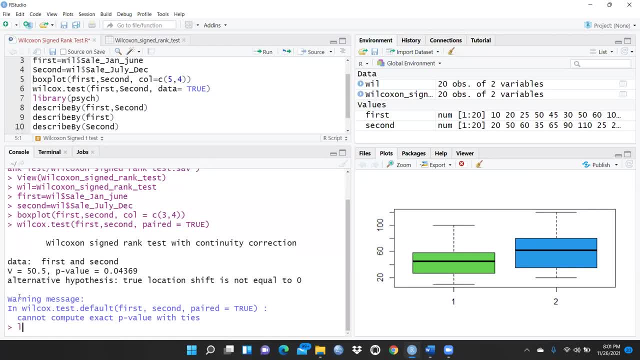 We have to check median values also. So for this purpose, simply, we need library, We need library and that package PSYPACKAGE right, and I have to select it. So the reason why it is important is that material is then bulbous in our All revitalizing systems. 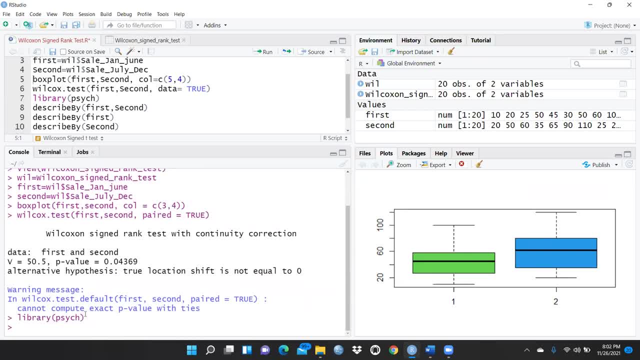 to press enter and because i i'm already having right this particular package and i have to use- there is the one one function, describe. if suppose you want to test individually, then you have to use this describe and let's say one by one, so i'm just writing first and i would press enter. so now,